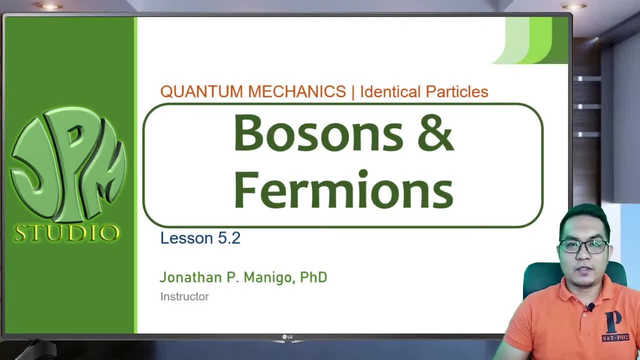 be introducing two types of particles. So in the previous lesson we have discussed about the two particle system. We didn't explicitly introduce or write the actual wave function. but we know that the time independent wave function depends on the position of both of the particles. So in the previous lesson 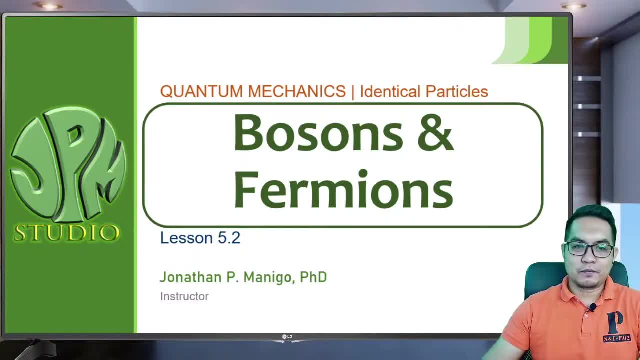 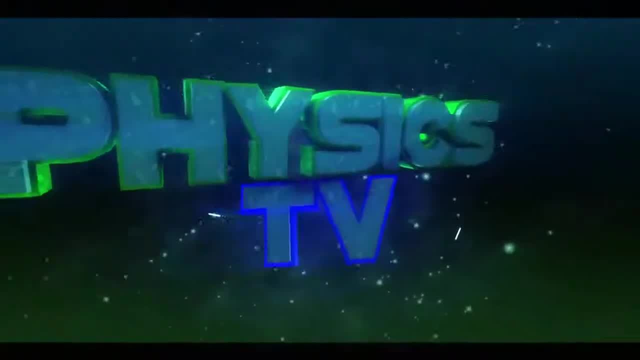 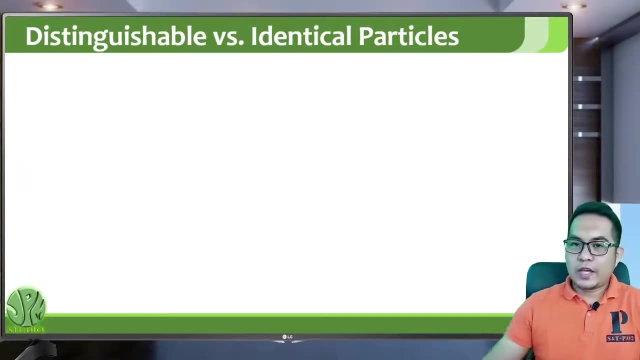 we have discussed about the two type of particles, The bosons and the fermions. So before we can write the wave function of a two particle system, we first need to identify if the particles can be distinguished from one another. So suppose there are two available states, state A and state B, and particle 1 is distinguishable. 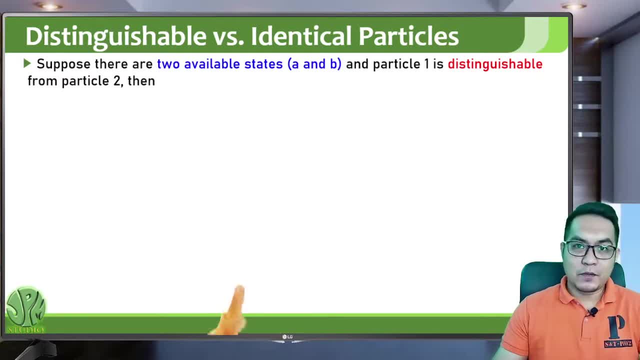 from particle 2.. You can clearly distinguish the first particle from the second particle, such as if you have an electron for particle 1 and you have a proton for particle 2, then they are distinguishable. Then if particle 1 is in state A and particle 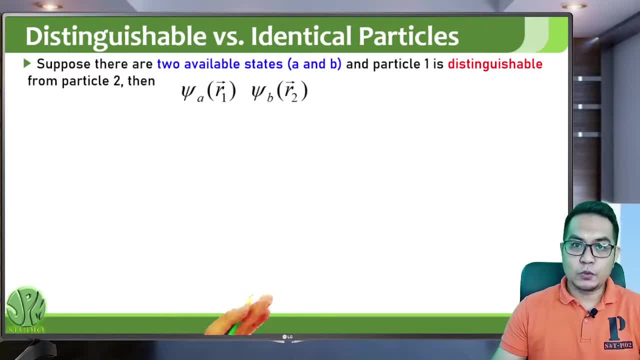 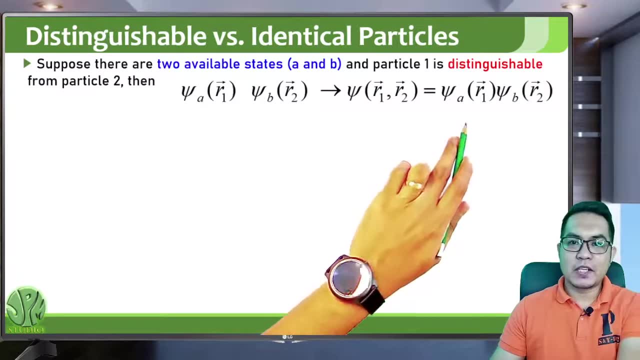 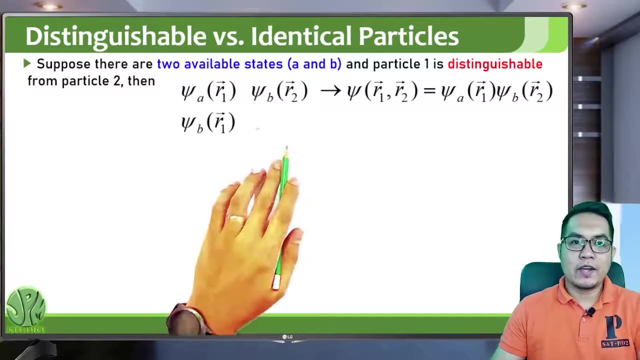 2 is in state B, then the wave function of the two particle system is just the multiplication of the wave functions. But there's another scenario: What if particle 1 is in state B and particle 2 is in state A- the reverse: Then we will also have this wave function. 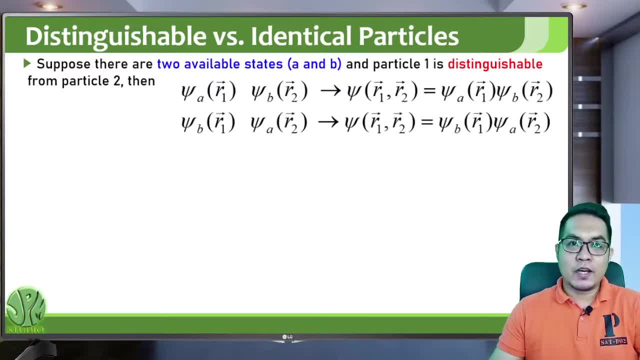 So that is the case. if you have distinguishable particles, You just multiply the two particles, multiply the wave functions, depending on which state a certain particle is. Now suppose the particles are identical, So you can no longer distinguish particle 1 from particle 2.. For instance, you have two electrons. All electrons are basically identical. 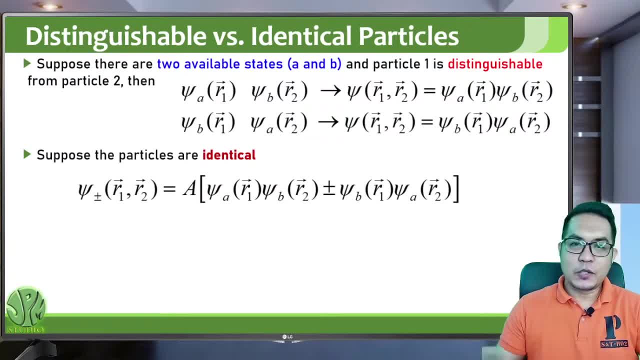 So the wave functions. since you can no longer know the wave functions, you can no longer know the wave functions. If you know which particle is in which state, then you have to take into account these two possibilities. What if the first is in A and the second is in B, or the reverse? Because 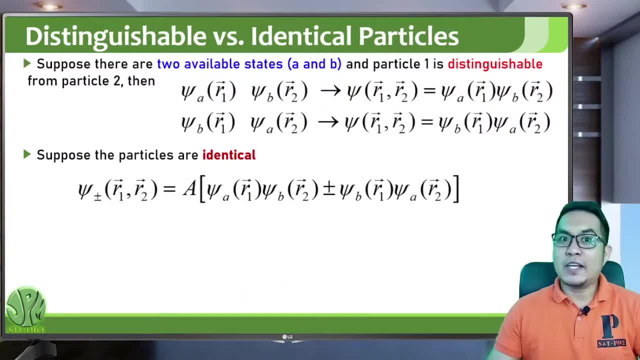 they're identical. You cannot know which particle is in which state, So you have to take into account the two possible states. So A here is just a normalization constant, And if you normalize this you will get. A is equal to 1 over square root of 2.. 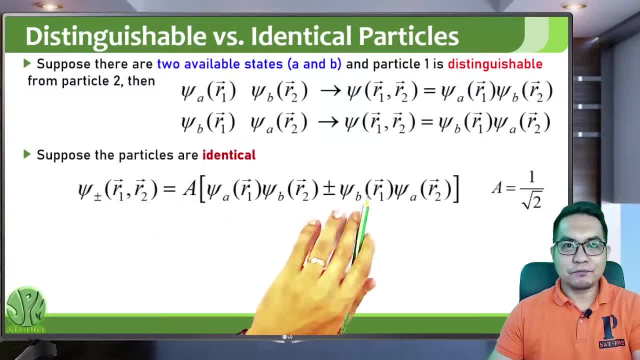 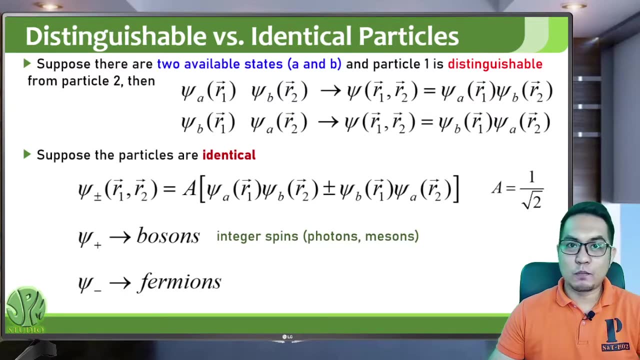 Now there's a plus and minus here. Either you add the possible combination or you subtract the possible combinations. You use the plus if you have bosons and you use the minus if you have fermions. So bosons have integer spins, such as photons, mesons, spin 1, spin. 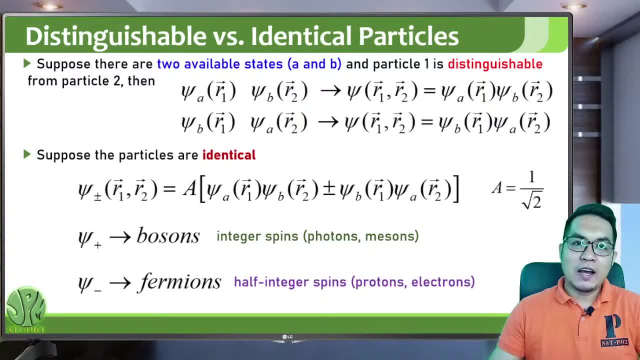 2, spin 3.. And Fermions are particles with half integer spins. So this is now bosons, and fermions are another way to categorize the final patterns. So that's it, Thank you, Bye. particles in terms of their spins. so if you have half integer spins, 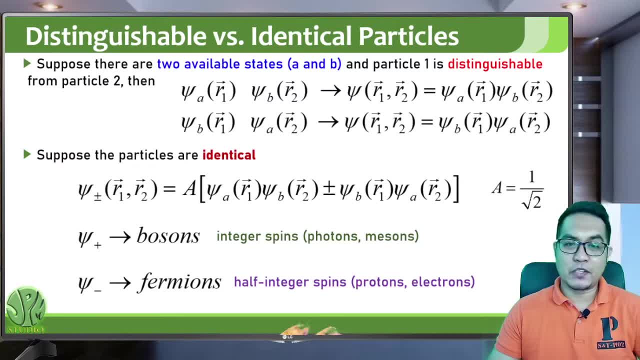 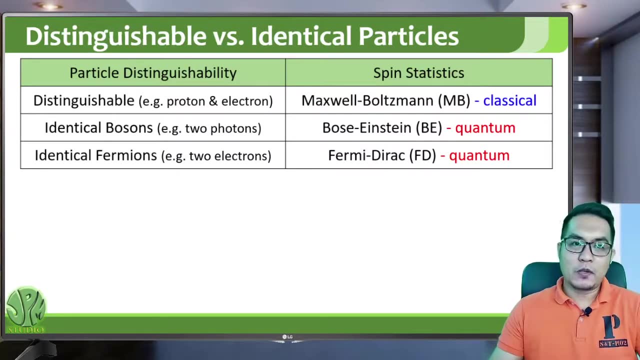 such as spin one half particles. we focused that one in the previous chapter, so those are permanent. so protons electrons are permanents. so this is now a table summarizing the statistics that you must use whether you have distinguishable or identical particles. so if you have distinguishable, 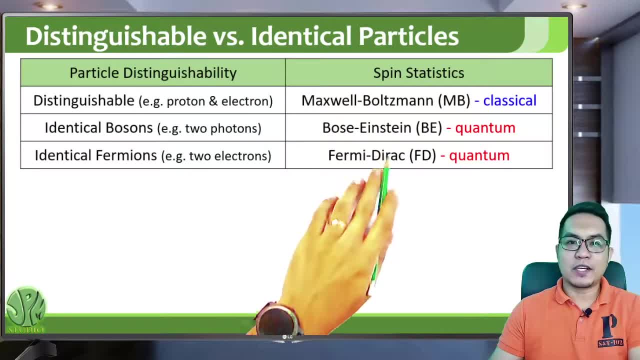 particles such as a proton and an electron, then you actually just use classical Maxwell Boltzmann statistics. but if you have identical bosons, so say two photons, so you need to use Bose-Einstein statistics, which is now a quantum statistics, and if you have identical fermions, such as two, 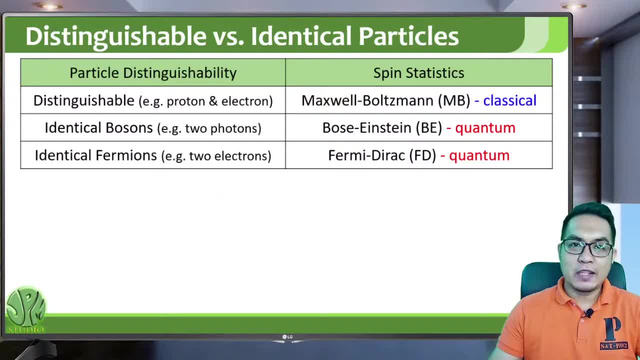 electrons, then you need to use the Fermi Dirac statistics, or which is also a kind of quantum statistics. so take note, even though a proton is a fermion and an electron is a fermion, but in this case they are distinguishable. so if you have two protons, that's the case of identical. 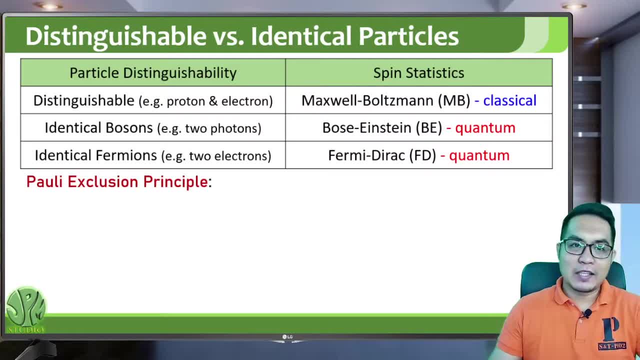 fermions if you have two electrons as a case of identical fermions. now, an additional rule for fermions- identical fermions- is that it's all about Pauli Exclusion principle. you have actually learned this in your basic chemistry. so identical fermions cannot occupy the same state. so if you have two electrons, 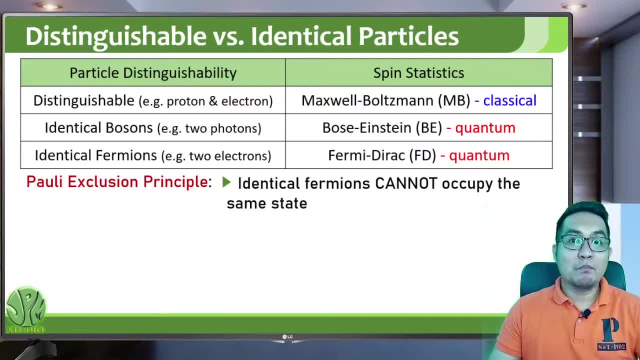 in a system, they cannot be in the same state. so for instance, in your chemistry, if one electron is spin up, then the other electron must be spin down. so for the symmetry requirement for bosons and fermions. so for bosons, identical bosons, if you interchange the 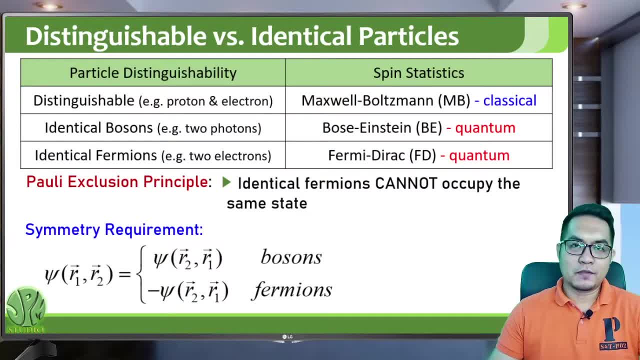 the position of the two particles, the two identical bosons, then the wave function will just be the same. But if you have identical premiums, if you interchange the position of the two particles, then the wave function becomes negative. So it's anti-symmetric. So, identical bosons, the wave function. 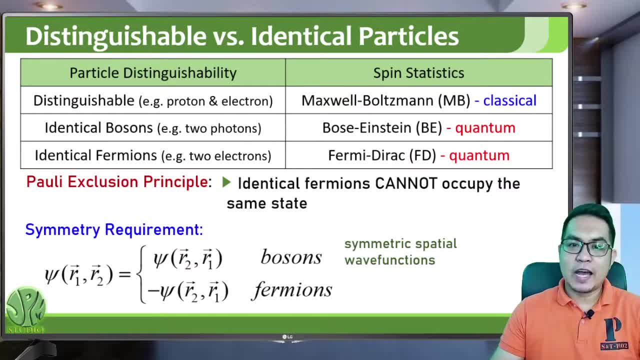 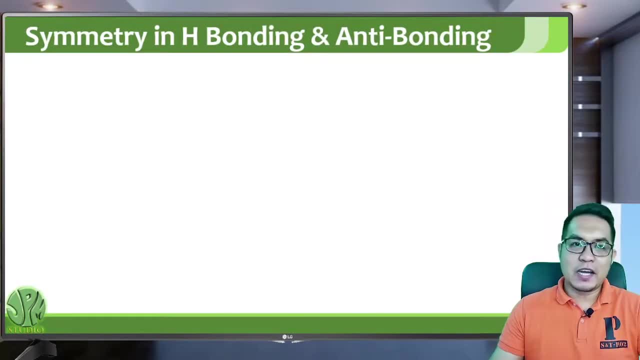 for a system composed of identical bosons have symmetric spatial wave functions or position wave functions, while a system composed of identical premiums have anti-symmetric spatial wave functions. So, as an example, let's consider the hydrogen bonding and hydrogen anti-bonding. So this is hydrogen. 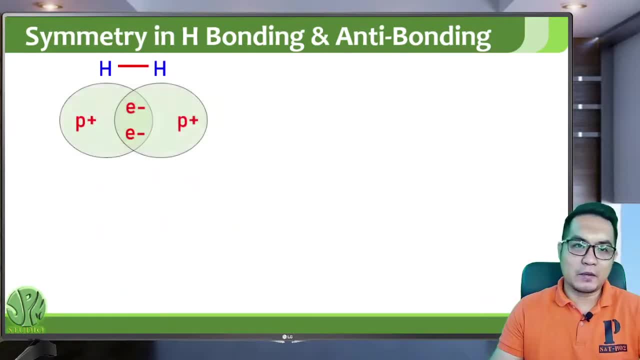 bonding, This is actually a symbol for covalent bond. So when in hydrogen bonding they actually share their, their, their, their only electrons to fill the orbital. So in the covalent bonding or hydrogen bonding, it's actually an attractive bond and the wave function of the 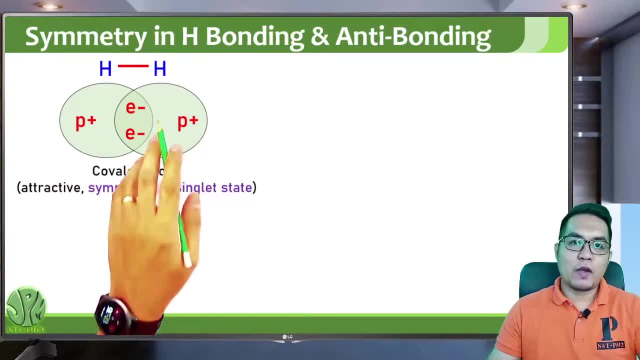 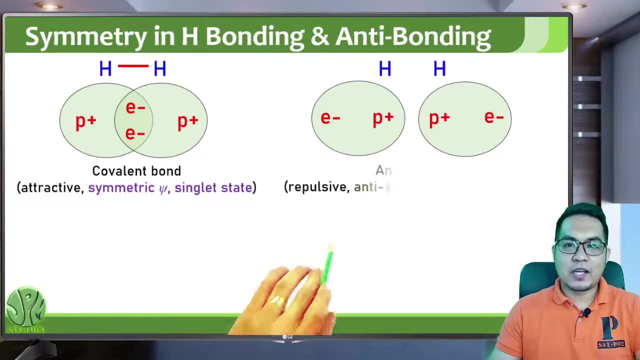 system is actually symmetric And the hydrogen actually is in the singlet state. So for anti-bonding it's actually repulsive and the states are actually anti-symmetric And the hydrogen atom here are actually in the triplet states. So if you will recall, the singlet state is this one. 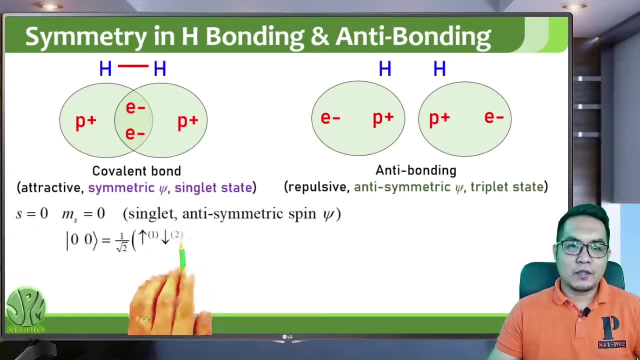 s is equal to zero, m is equal to zero. So you will notice that the singlet state is actually anti-symmetric, because if you interchanged one and two because of the negative sign here, minus sign here, which is a subtraction, then you will get a. 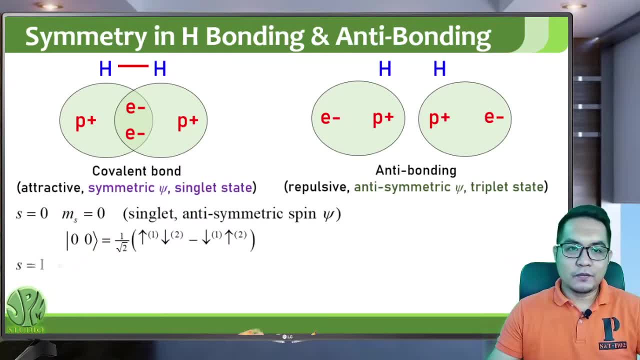 negative wave function or negative state. On the other hand, triplet states are symmetric. whether you exchange one particle one and particle two, it's still the same wave function. Now, how does this happen When, if in anti-bonding, the hydrogen are in triplet state and the triplet 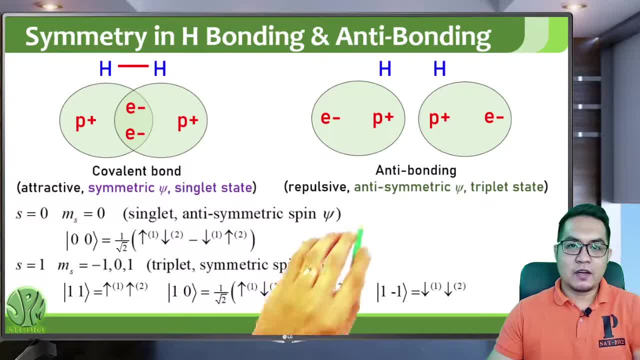 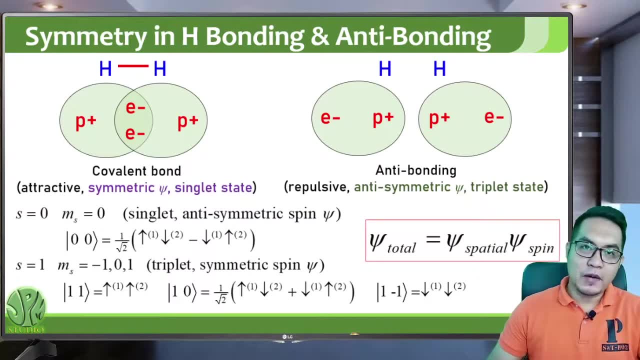 state have symmetric spin wave functions, but the total wave function of the system is anti-symmetric. So you have to recall again that the total wave function of a system is a product of the spatially function and the spin wave function, The spatially function. 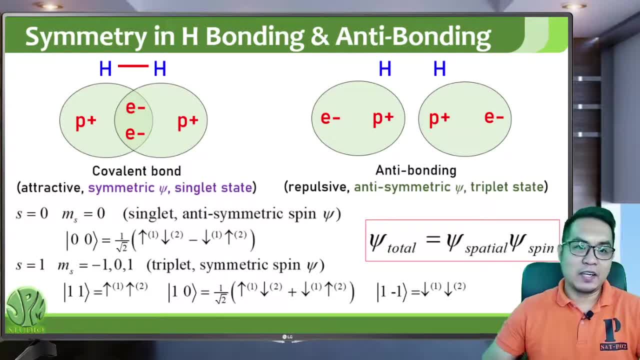 for the hydrogen atom is actually an anti-symmetric And if you multiply it with the spin wave is an anti-symmetric spin wave function, which is the singlet state. then you get a symmetric wave function for the system. And if you multiply the anti-symmetric, 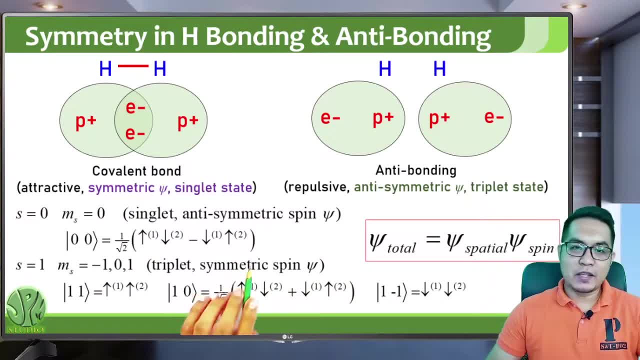 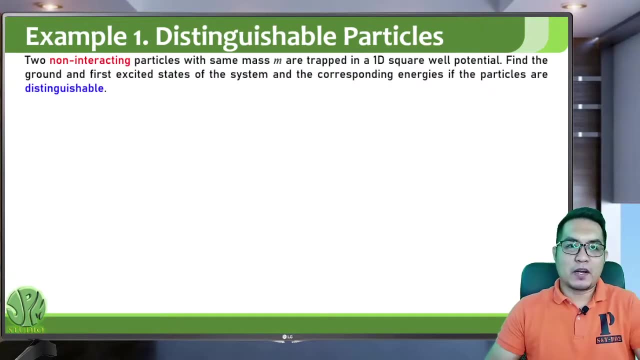 spacial wave function. with the symmetric spin wave function, then you will get an wave function which corresponds to anti-bonding. So let's now have an example. So example one is distinguishable particles. So you have two non-interacting particles. So let's emphasize that they are non-interacting, so that the 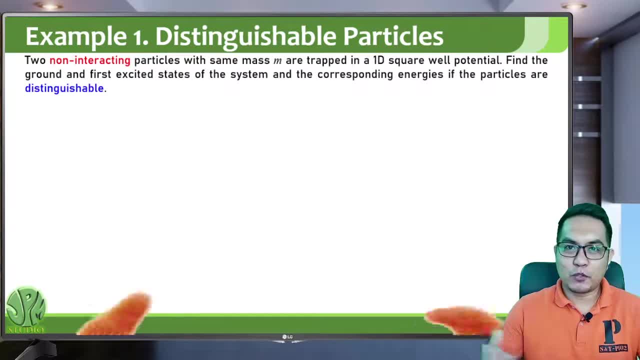 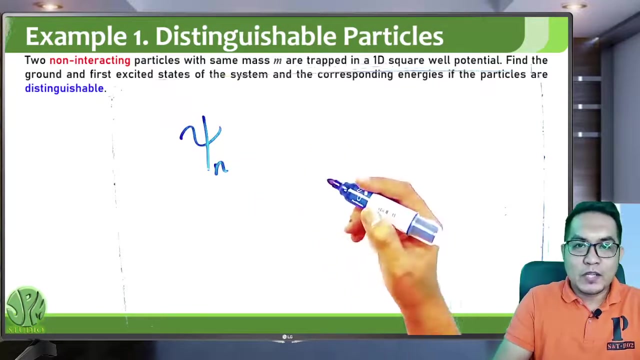 energy is purely kinetic energy. They have no potential interaction. potential energy. So two non-interacting particles with the same mass m are trapped in a one dimensional square well potential. So, if you will recall the one dimensional square well potential, the wave function for a particle trapped in a one dimensional square well potential is given by 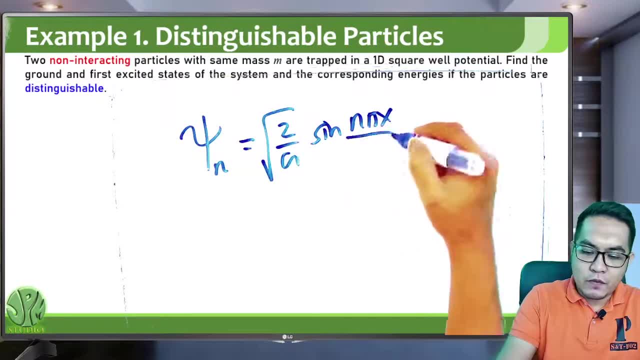 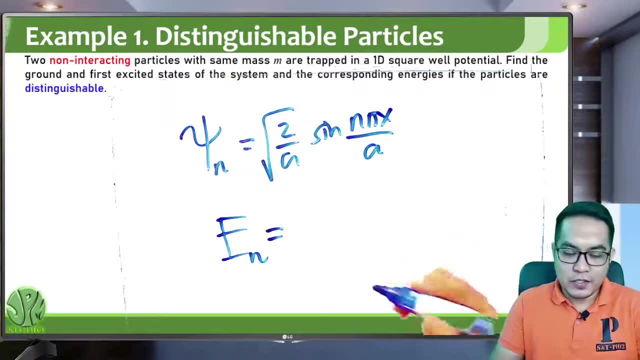 sine n, Pi, x over a And the energy levels for a particle trapped in an infinite square. well, potential, One-dimensional, infinite square. well, potential potential is n squared pi squared h, bar squared over 2 m, a squared that one. so you are then asked: 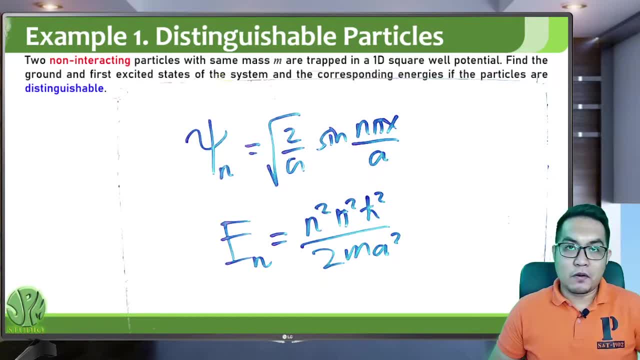 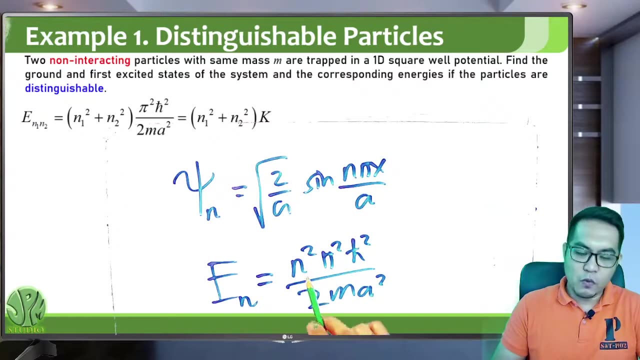 to find the ground and first excited states of this two particle system and the corresponding energies. if the particles are distinguishable, okay. so if the particles are distinguishable, then the total energy is just the energy of particle, one which is n1, pi squared, h bar squared. 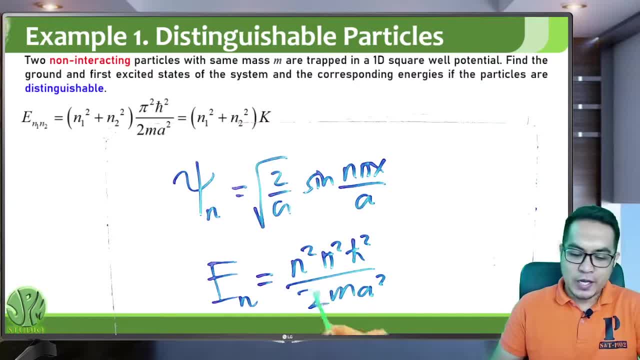 over 2 m a squared, plus the energy of particle two, which is n2 squared pi squared h, bar squared over 2 m a squared, and you will get this result. we will just let this constant pi squared h bar squared over 2 m a squared as a constant k for that. so it's just n1 squared plus n2 squared k. 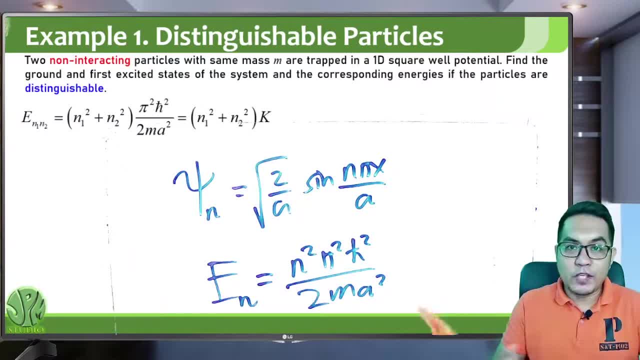 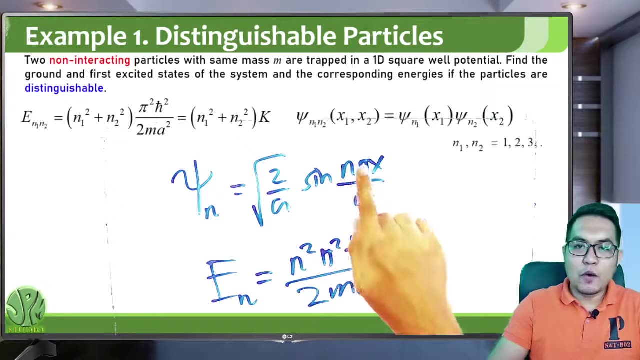 so that is the energy, general energy of the two of these two particle system for the states, since they are distinguishable. so it's just a product of the the two states. so the state of particle one, state of particle two. take note that n1 and n2 here. 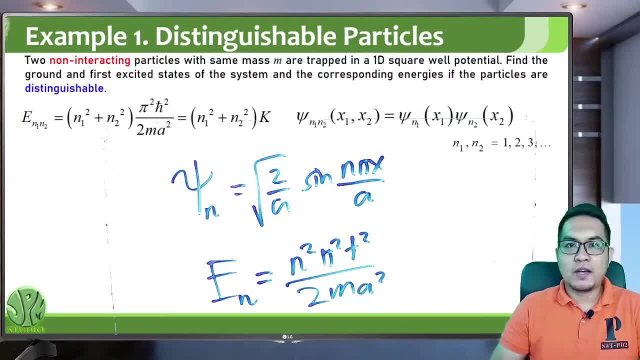 can have values from one, two, three, four and so on. so particle one could be in state, psi one. particle two could be in state also, psi one, psi two, psi three, psi four and so on. so this is the general two particle state. it's the general energy. so we are asked to find the ground state and the 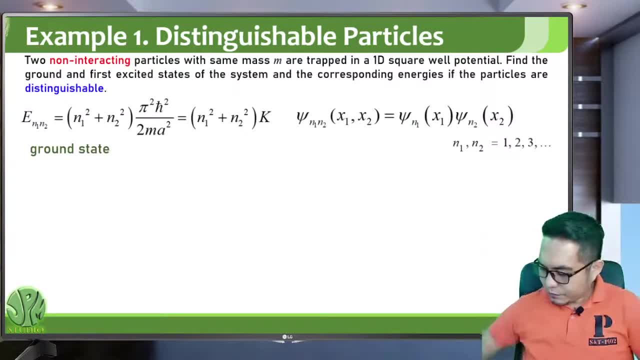 first excited state. so we first start with the ground state. so the ground state for the ground state we use the first solve for the ground state: energy. so what is the ground state energy? it's the lowest energy of the system. so what's the lowest value of this? so this happens when n1 is equal to one, the smallest value of n1 and n2, which 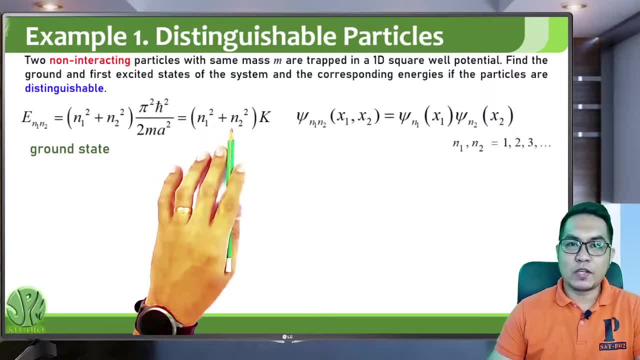 is one and n2 is equal to one. so you have one squared plus one squared, you have two k. so that's the ground state: energy, two k and what is the corresponding state. so n1 is equal to 1, n2 is equal to 1, so you will have: 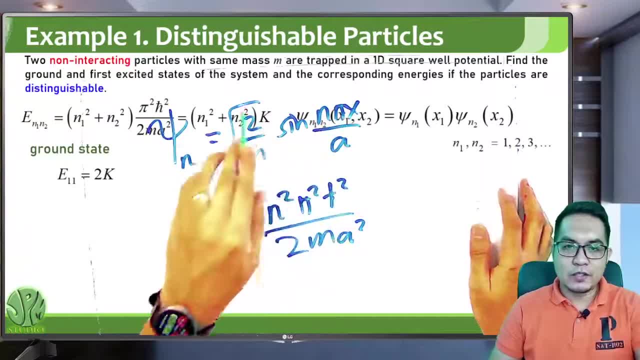 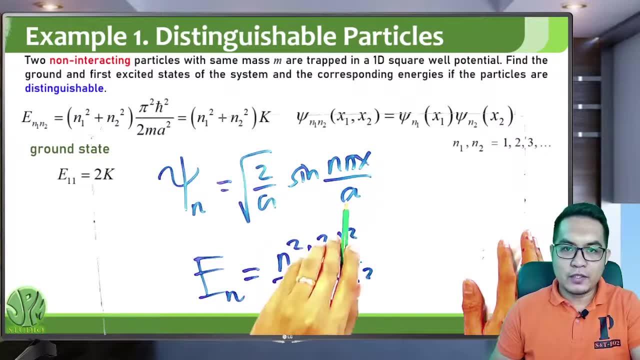 for n1 and n2 is equal to 1, so that the form, the wave function is square root of 2 over a sine n1, pi x1 over a multiplied by wave function for x2, which is also in state, psi n1. so you have that: multiply the two-way function and you will get this result. so you: 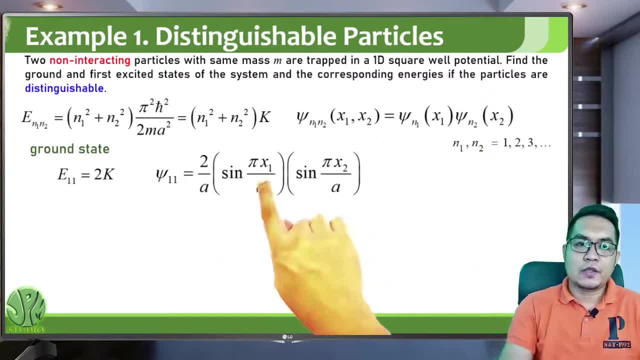 have 2 square root of 2 over a, so you will get 2 over a. so sine pi x1 over a, sine pi x2 over a. so n1 and n2 are both equal to 1. so this is the ground state. so how about the first excited? 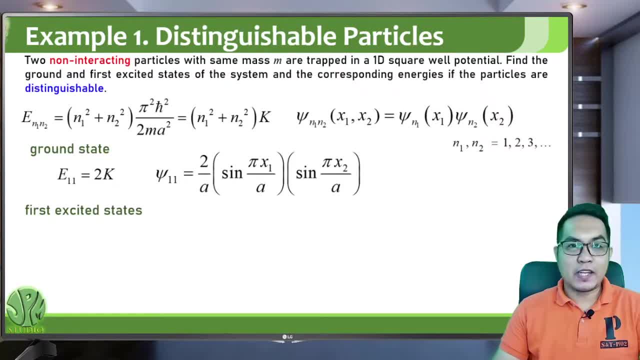 state, so the next energy corresponding to the next energy line. so this happens when n1 is equal to 1. so this is the ground state. so how about the first excited state? so the next, n1 is equal to 1 and n2 is equal to 2. so 1 squared plus 2 squared, you will get 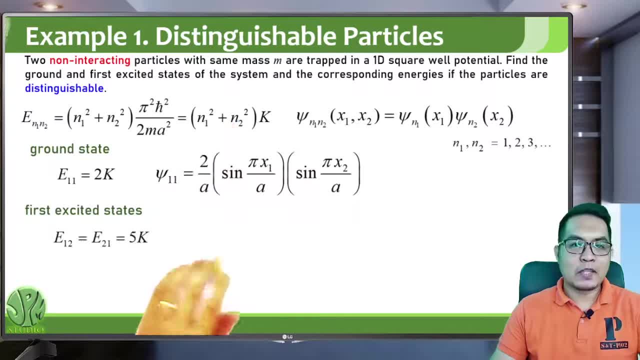 5k, but that's also the same for when n1 is equal to 2 and n2 is equal to 1. it's still the same energy, 5k and the first excited. so this means that there will be two first excited states: psi 1- 2 and psi 2- 1. so just multiply the two-way function. 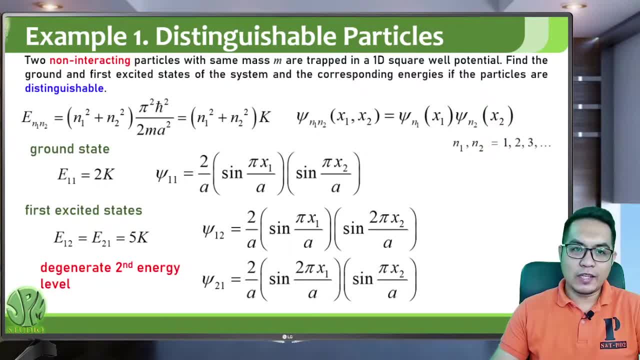 so psi 1: 2 and psi 2: 1. so we call this energy level as a degenerate energy level. so the ground state is non-degenerate, meaning one energy level, one state. but the second energy level, which corresponds to the first excited states, is no longer non-degenerate, it's actually degenerate. 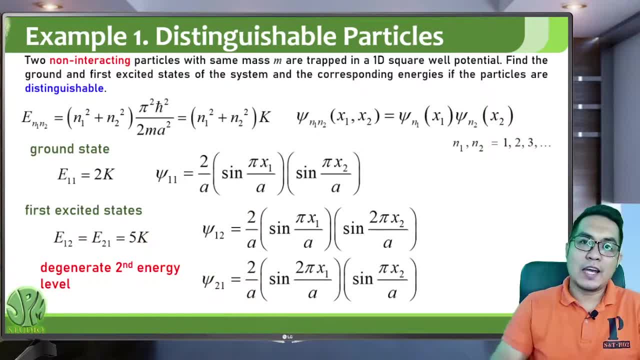 there are two states corresponding to this energy level: 5k. so psi 1: 2 and psi 2: 1. so that's all that. those are the first and this is the first excited ground state, and these are the first excited things. so let's have another example. 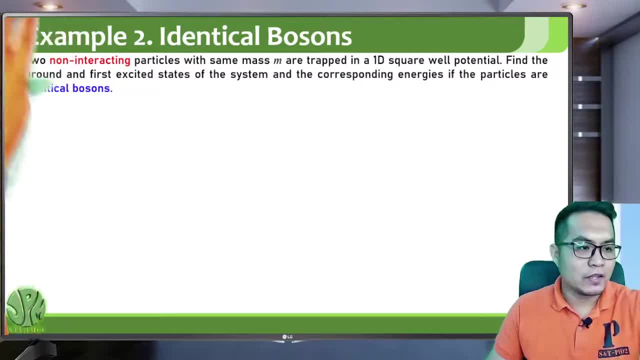 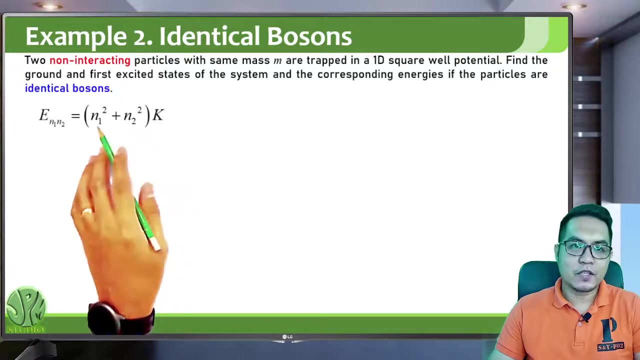 it's just a similar problem, but now instead of distinguishable particles we now have identical particles, and they are bosons, identical bosons. so the same problem: find the ground and first excited states of the system and the corresponding energies. so they will have the same corresponding energy. so energy of particle 1 plus energy of 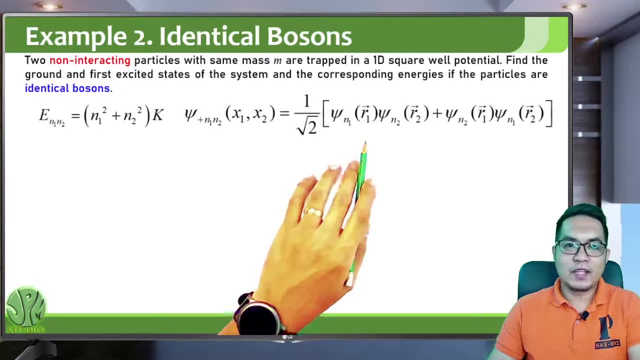 particle 2, but the state is now this one. you now take into account the possible combination. so what if particle 1 is in state n1, particle 2 is in state n2, or what if particle 1 is in state n2 and particle 2 is in state n1? so you take all the possible combinations and you can. 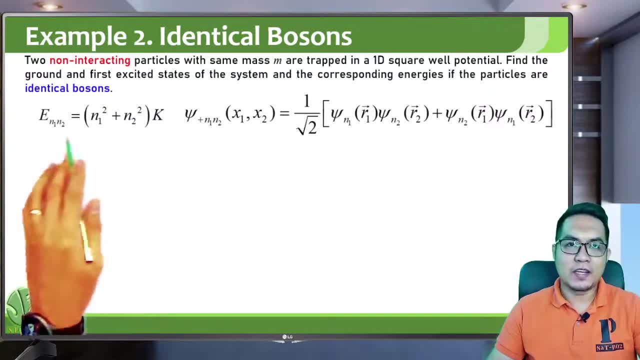 take all the possible combinations. so this is the general generic energy of the system, it's the general state of the system. so let's first start with the ground state. so again, we first solve for the energy before we solve for the ground state. so again, the ground state is when n1 and n2 is. 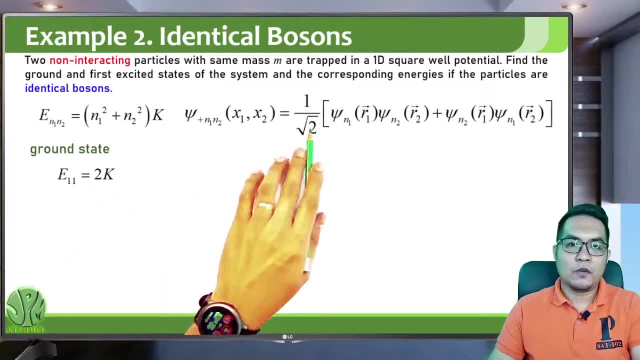 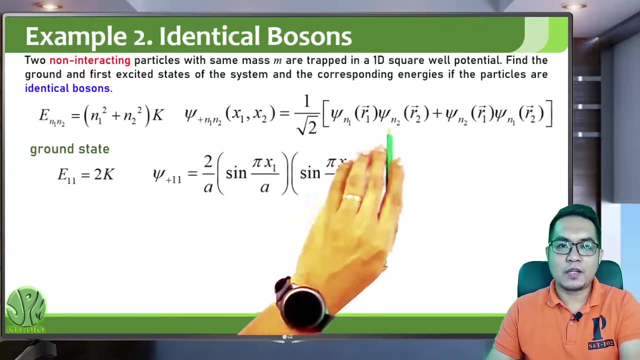 equal to 1, so it's still 2k. now, when n1 and n2 is equal to 1, use this equation and you will get this one. so use this. use this equation. look for psi 1 r1, psi 2, psi 1 r2, then psi 1 r1, psi 2 r2. so 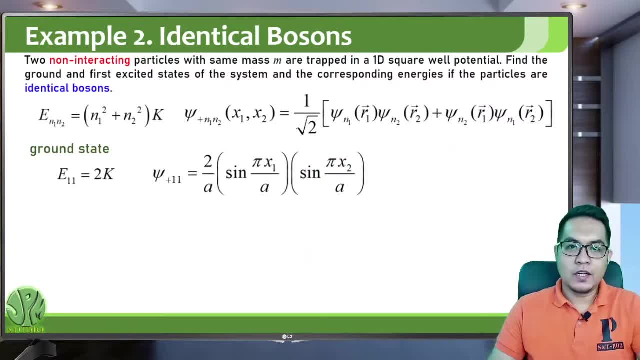 basically, you just add the two and then you will get this result. so basically it's the same state as the distinguishable case. basically, just multiply the two. uh, just multiply. the effect is just multiplying the two-way functions. so how about the first excited state? now, similarly with the distinguishable case. 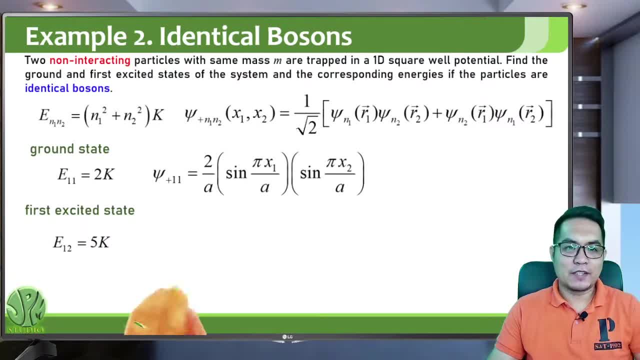 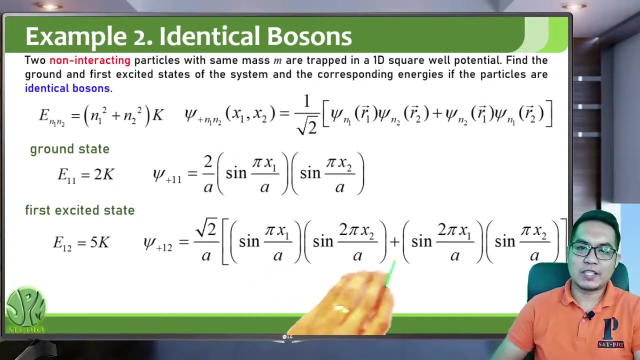 this first excited state, energy is 5k. but now, since in the formula we already take into account the possible combinations, then there will be no uh state. 1, 2 and 2, 1 are basically uh. in this uh state sign 1, 2, because this is 1, 2, this is 2: 1. 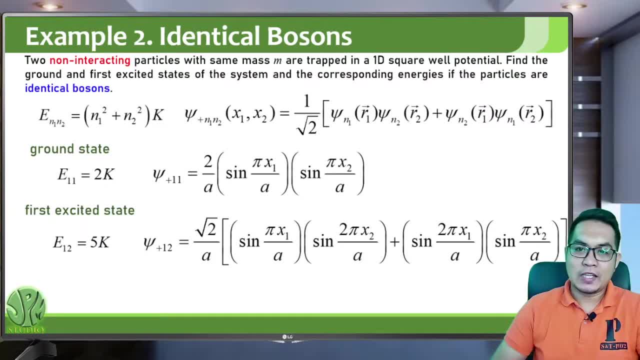 we already take, took into account the possible combinations. so this: from this formula you get this: uh result again in solving the wave functions. for each of the energy energy or for each of the state use, the single particle will function. so the only difference now the identical bosons case with the distinguishable case is: 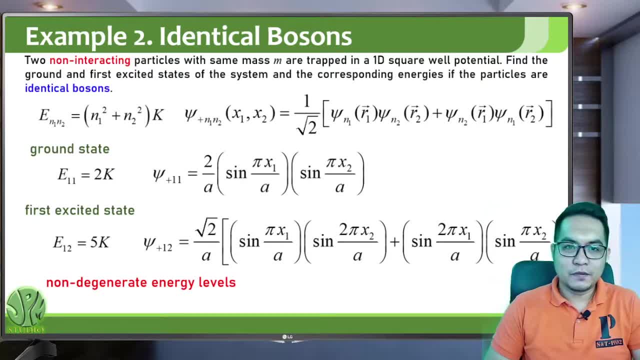 that the second energy level is also non-degenerate because you already want to undo one are basically in one state, are taken into account in one state, the side plus one. so this is actually the quantum effect. so if you go to quantum mechanics, most of the or the energy levels actually become non-degenerate. 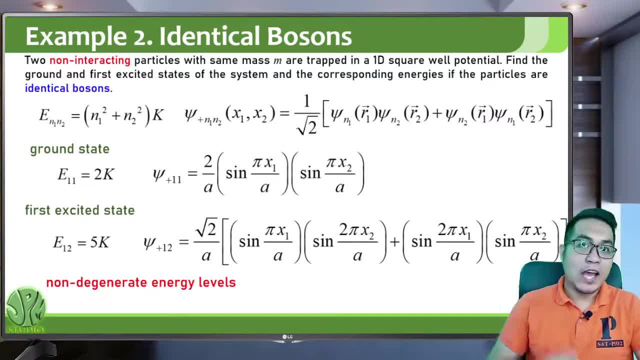 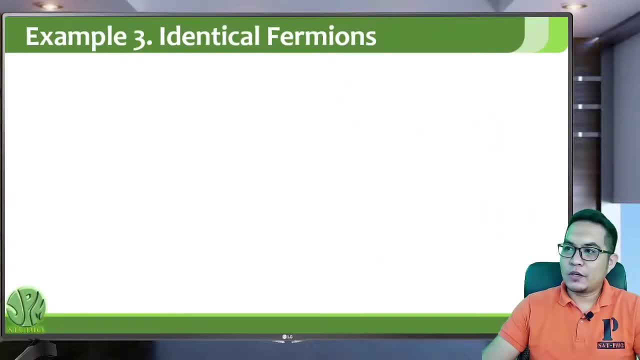 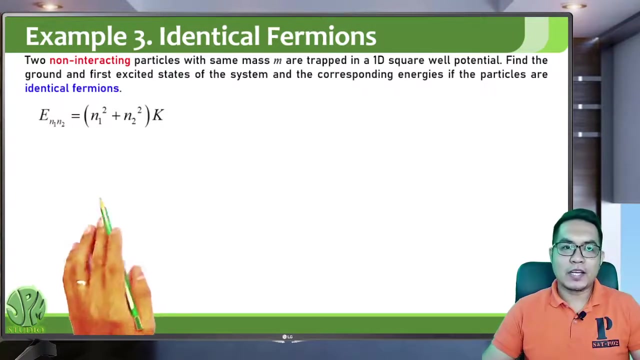 meaning there's only one state per energy level. so that what's happened when you go to the quantum realm? so how about the case for identical fermions? same problem: find the identical, find the ground and first excited states if the particles are identical fermions. so again the same general total energy, energy of particle. 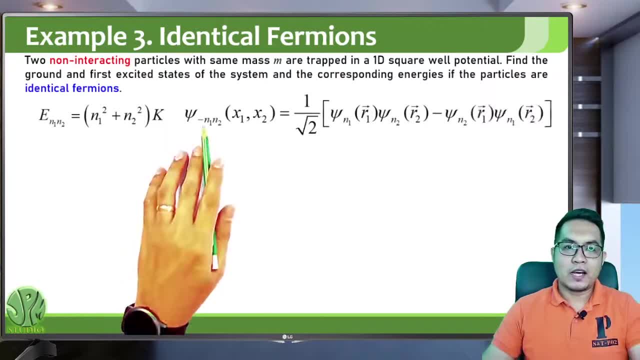 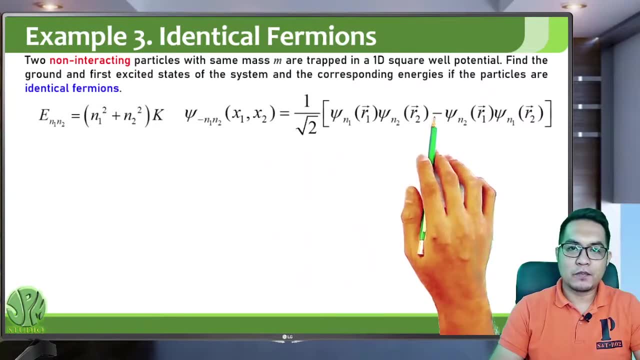 one energy of particle two. but the general state of the two particle system will now be this one. so it's now a minus because this is now identical fermions. so for the ground state you need to take into account Foundley exclusion principle, so no two identical fermions can occupy the same state. 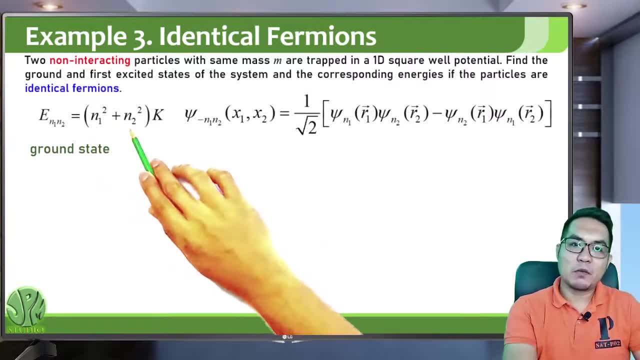 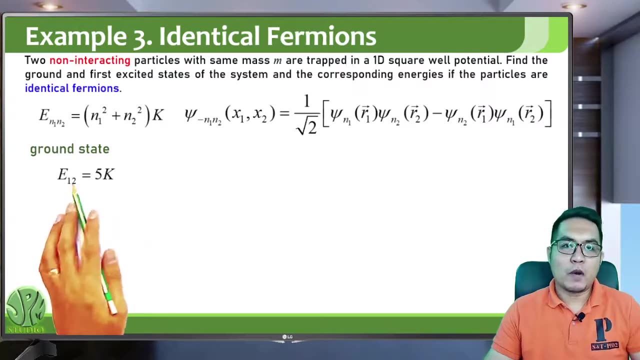 meaning: anyone cannot be equal to and to must not be in the same state. you must not be in the same state psi 1.. Therefore the ground state energy will be 5k, That is, when one particle is in state psi 1, the other particle is in state psi 2.. Take note, we don't know. 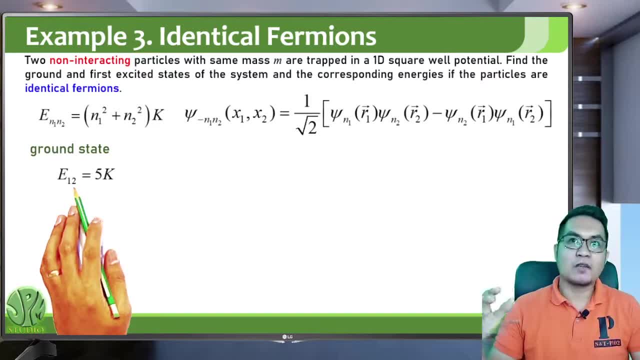 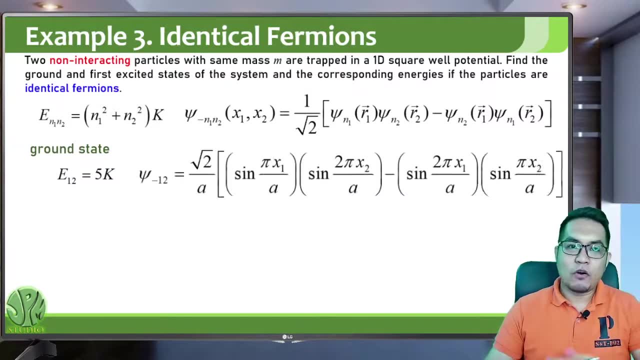 which particle is in which state. but we know that one of the particles is in state psi 1 and one of the particles is in state psi 2. And we take all the possible scenario combinations and we obtain this ground state. This is now the ground state of two identical fermions trapped. 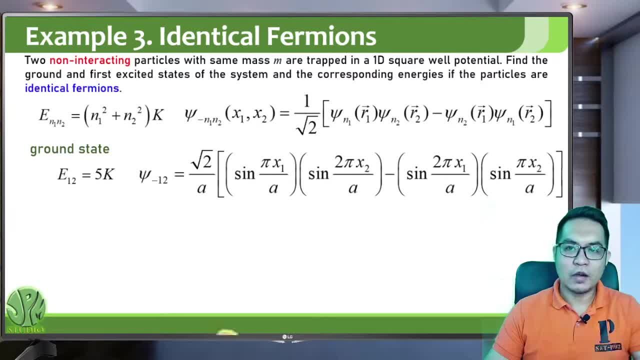 in a one-dimensional square potential. Now for the first excited state. again, n1 and n2, or the particle 1 and particle 2, cannot be in the same state. So therefore 2, 2,, n1, 2, 2 is not an option. And the next energy level? 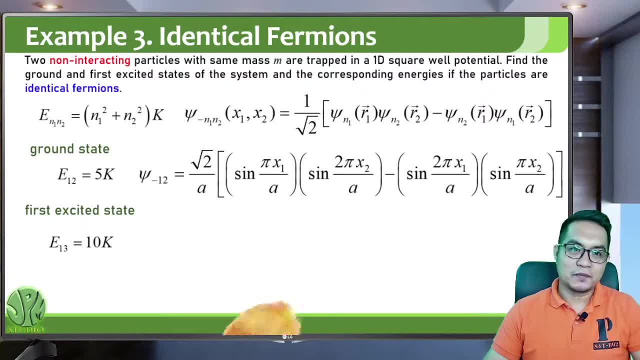 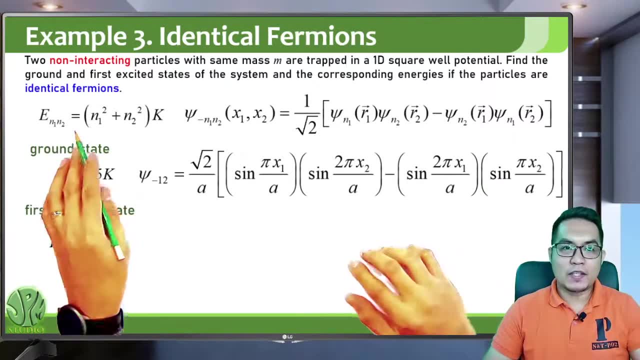 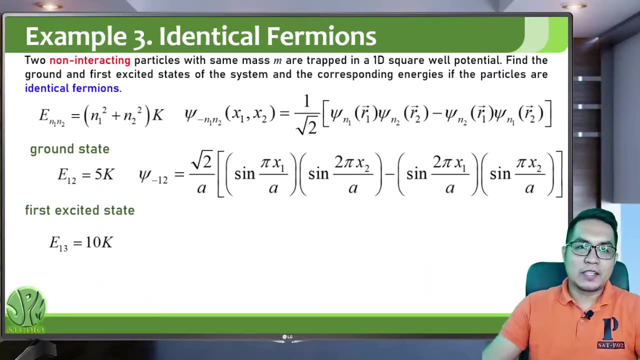 will be 1, 3.. So one particle is in state psi 1, the other particle is in state psi 3.. So 1 squared plus 3 squared you will get 10k. So that is the first excited state energy level And using the 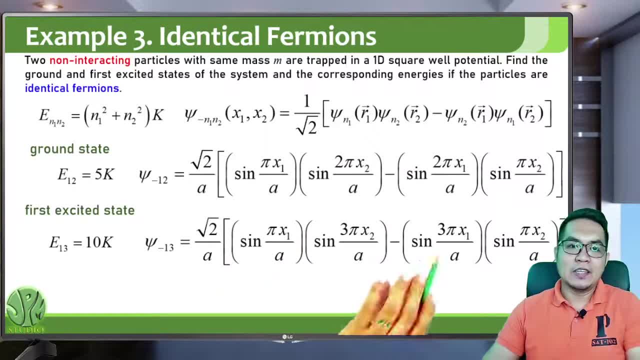 same formula. this formula: you get the first excited state for a two-particle fermion and the second excited state for a two-particle fermion. And take note, the energy levels are also non-degenerate because this is now the quantum-a-quantum effect. So when you go to the 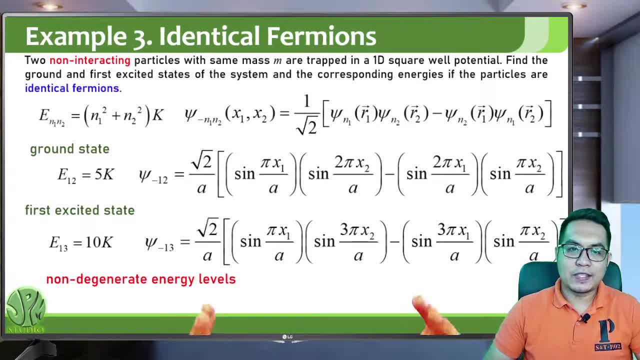 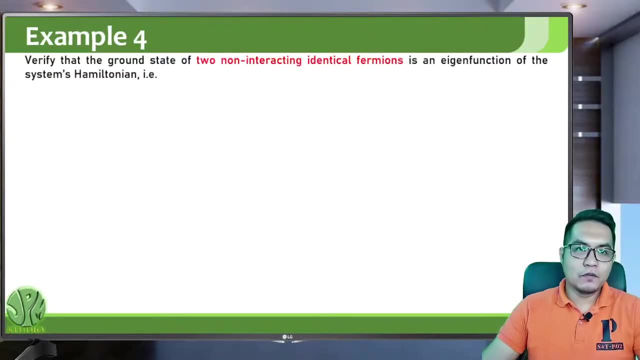 quantum realm. when you make your system very, very small and they are composed of identical particles, then the energy levels become non-degenerate. So for our last example, we can verify that the ground state is in state psi 1, and the energy levels are also non-degenerate. 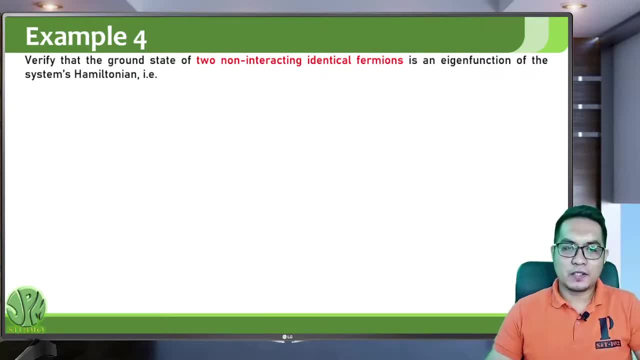 So the ground state of two non-interacting identical fermions in an infinite square-wheel potential. it's actually a continuation, is an eigenfunction of the Hamiltonian. So the Hamiltonian acting on psi minus 1, 2, the ground state of the identical fermions in 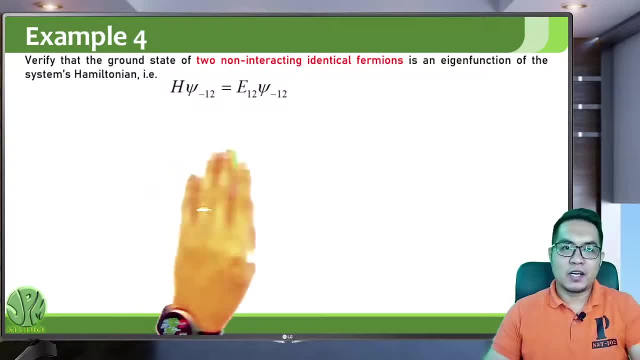 one-dimensional infinite square-wheel potential obeys the time-interferon state. So the ground state of the identical fermions in one-dimensional infinite square-wheel potential is actually a continuation, is an eigenvalue equation. So if you can show that you obtained this, 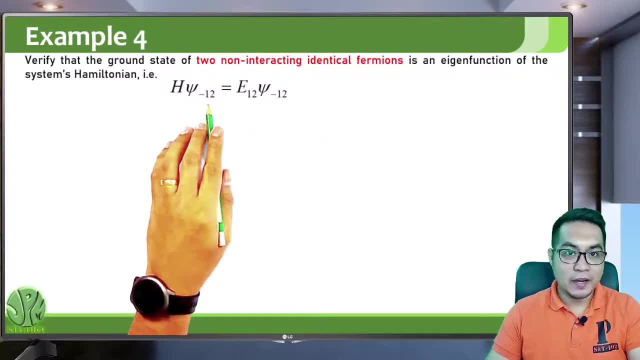 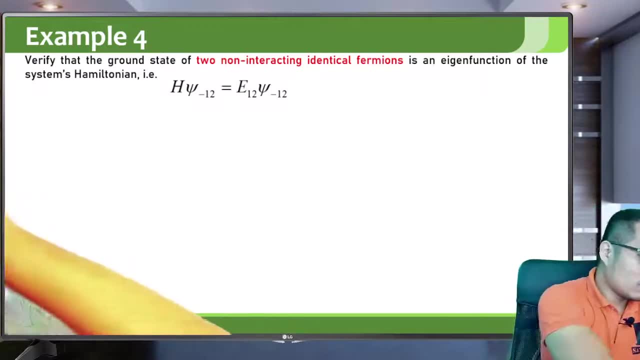 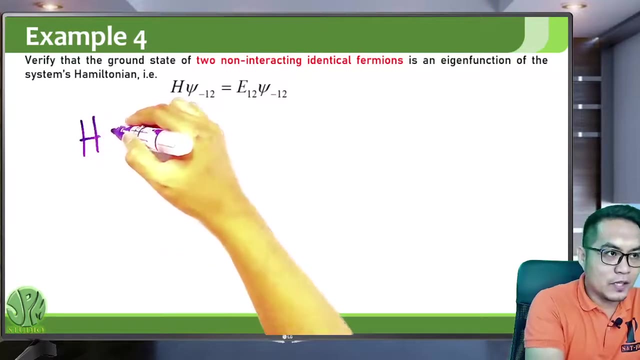 one, then this means that psi minus 1, 2 is an eigenfunction of H, the Hamiltonian. So I will not be solving this totally, I will just discuss the main concepts used here. So the Hamiltonian of the system is just the kinetic energy of a set of two elements and the Hamiltonian is the kinetic energy of a set of two elements. So that means the Hamiltonian of the system is just the kinetic energy of a set of two elements. And if you can see the Hamiltonian of the system, if you can see this, that is the Hamiltonian of the system. 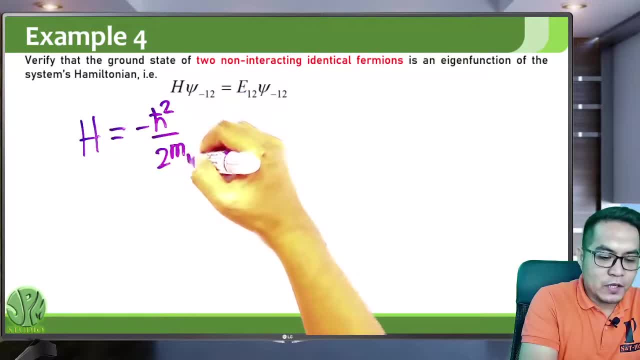 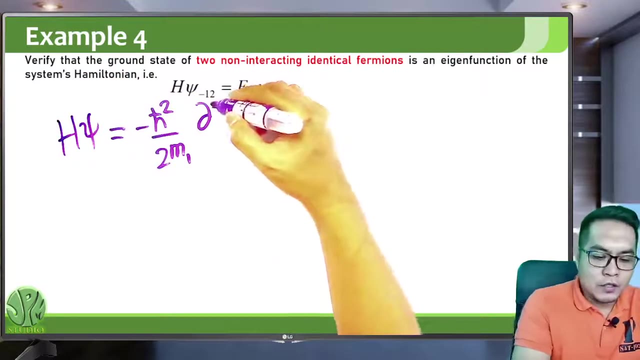 particle 1, so we'll get h by square root of 2m, since this is just one dimension, so you will just have psi. I will just use h of psi. so kinetic energy of particle 1 acting on psi, psi minus 1, 2. 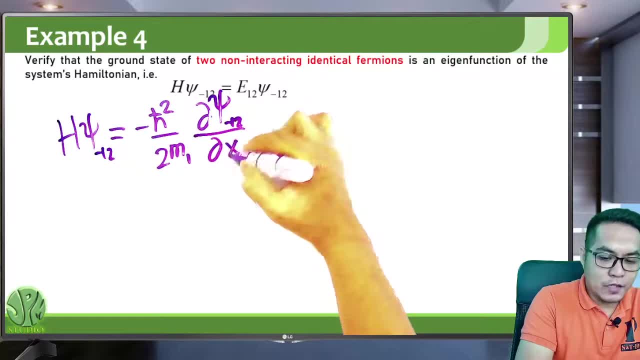 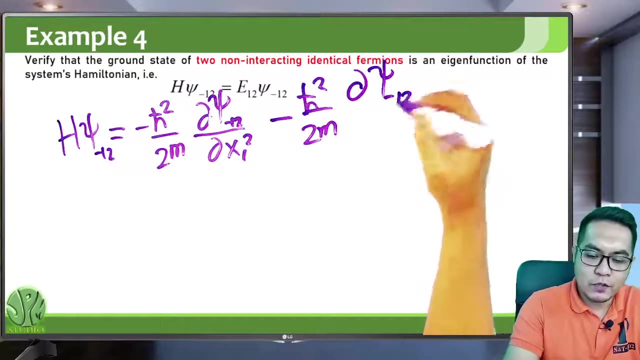 with respect to x1, squared plus the kinetic energy, which is negative. h by square root of 2m: 2. since they are identical, they have the same mass: h by square root of 2m, partial of psi of minus 1, 2.